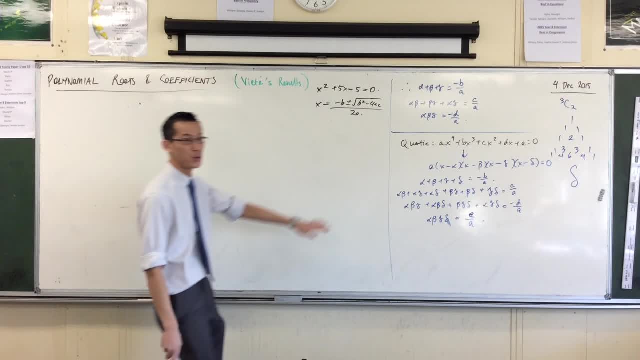 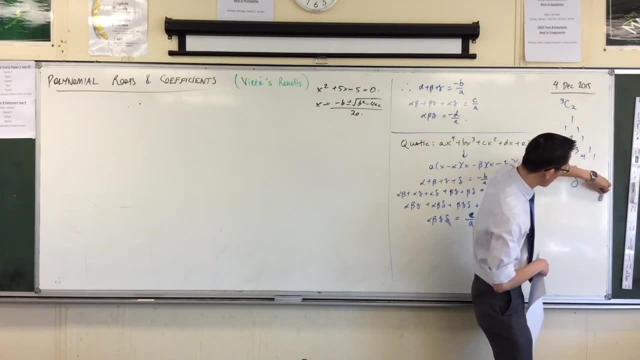 But as you add layers of complexity, as you go to say, the cubic things get a little more difficult. So thank you for my helpers who gave me BluTack. right, I'm doing it this way because I don't want to write out the cubic formula, because this is what the cubic formula looks like. 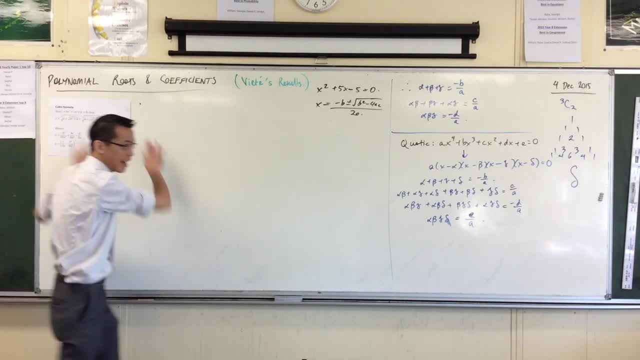 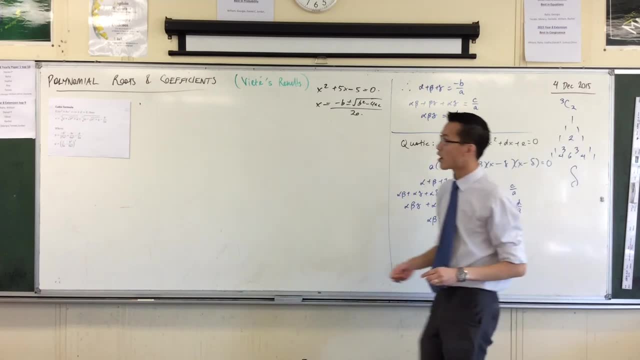 Now just look at it for a second and contemplate what it's doing. It's doing the same thing that the quadratic formula is doing. okay, It's saying: look, you want to start with a general cubic right: a x cubed plus b x cubed. blah, blah, blah. 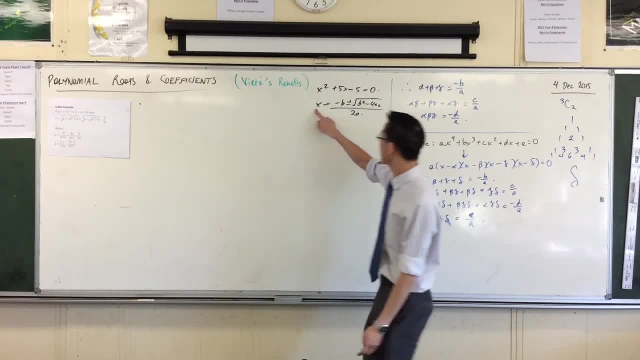 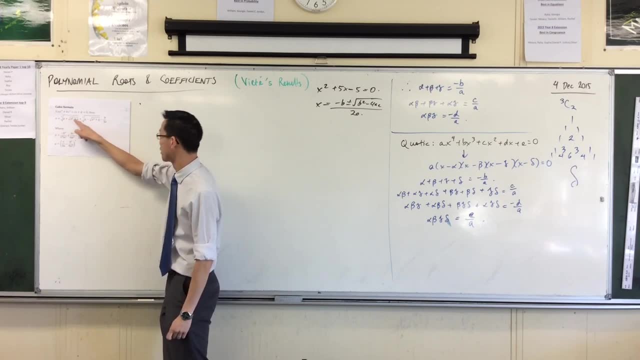 Right, It's saying: well, tell me what x is, Tell me what x is. There were two of these. There should be three of these. right Now. you look at this and this looks bad enough. You've got cube roots of square roots of blah, blah, blah. 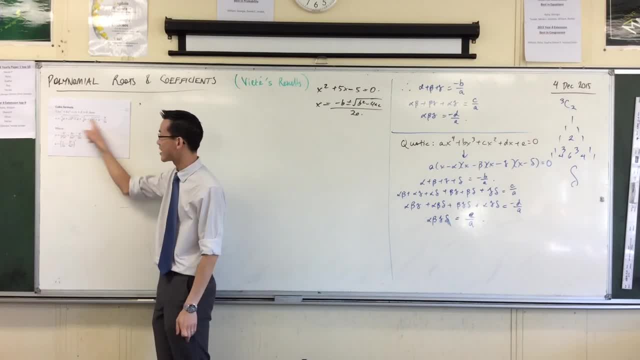 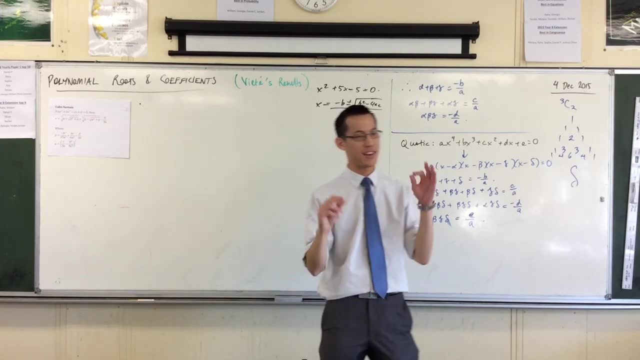 That looks bad, But actually it's even worse, because all of these things underneath the square root, if your eyesight is not that good, right, All of these things are also disastrous things themselves, right? It's just, it's really terrible, okay. 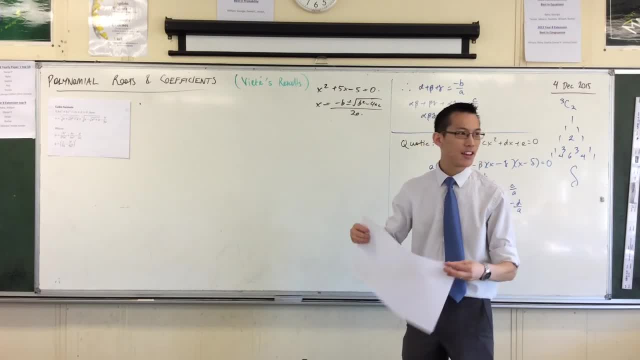 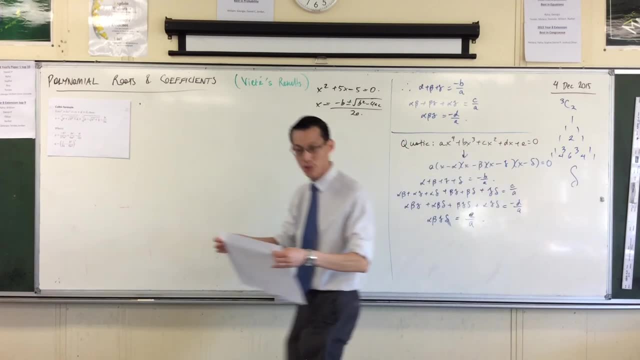 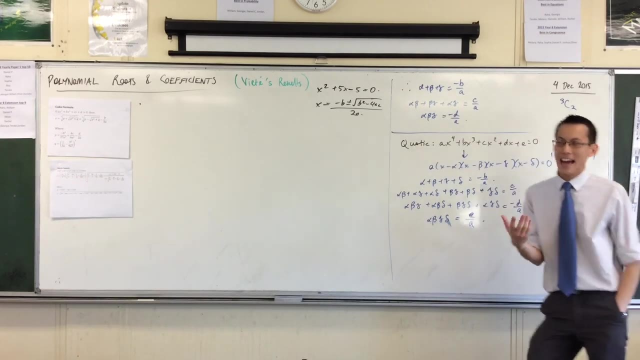 Now the cubic formula is bad. We went from the, We went from the quadratic to the cubic and that's what happened, right, When you go to the quartic Now, what basically happens is remember how I said here for the cubic formula. okay, 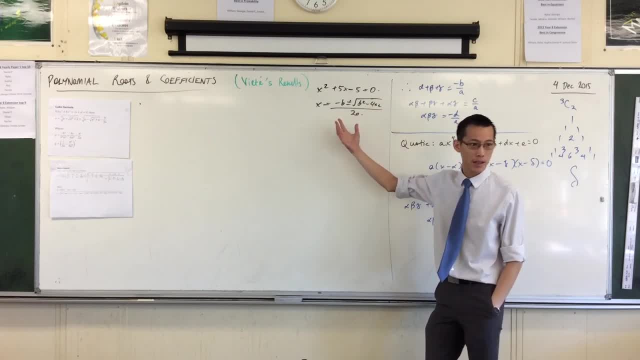 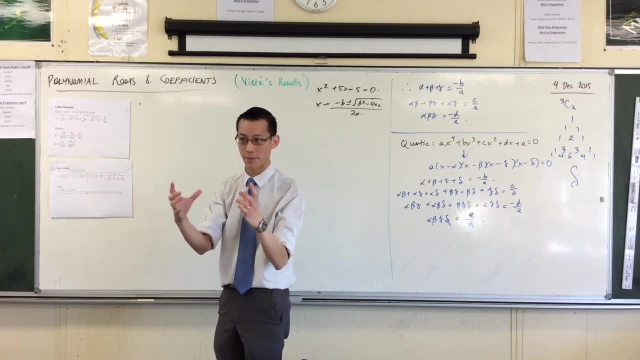 In the quadratic, the building blocks are just a, b and c- okay. When you move up to the cubic, the building blocks become things that themselves are the size of the quadratic formula. okay. When you go to the quartic, the building blocks are things that are the size of the cubic formula. okay. 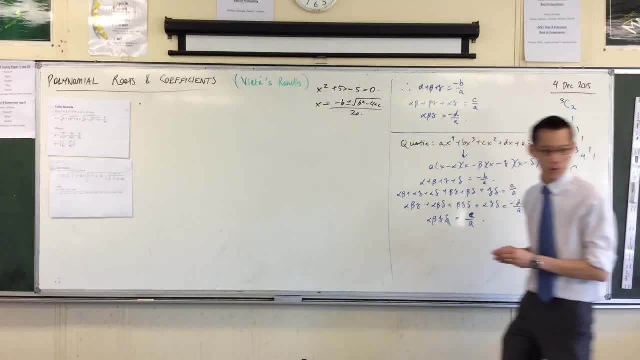 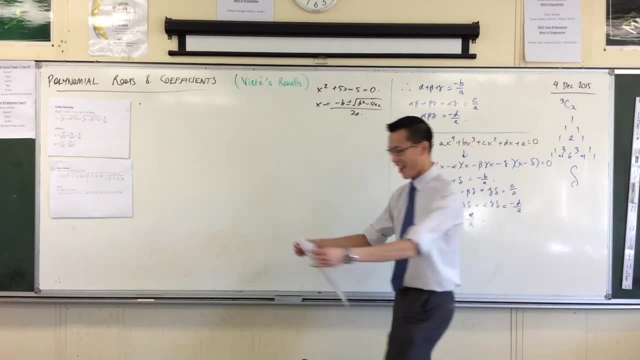 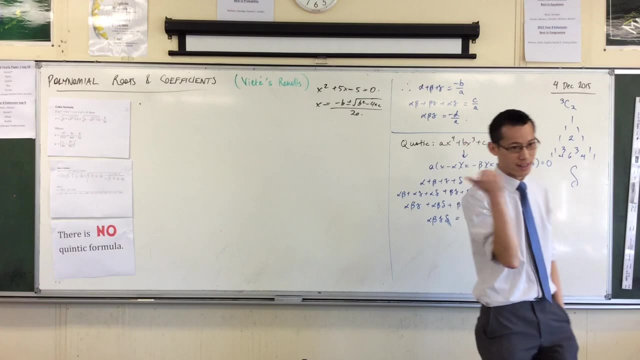 Now here's my favourite: one right, Because after three and then four comes five, right. So this is this is this is my favourite. By the way, This is my favourite Now. um cubic is three, quartic is four, quintic is five. 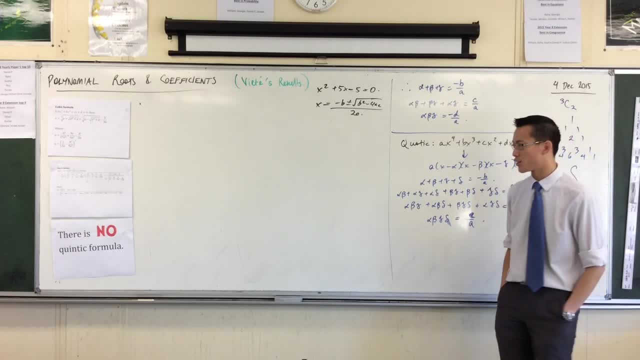 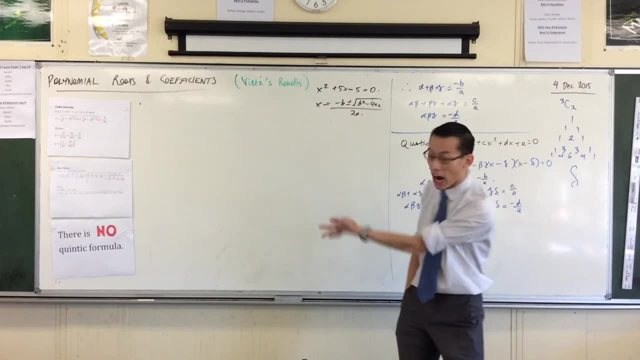 Now when I say there's no quintic formula, notice I don't say Um, we just haven't found it yet. okay, What's astonishing is it's been proven that you can't find a quintic formula or a hext or hepti or I don't know for any degree higher than four. right, 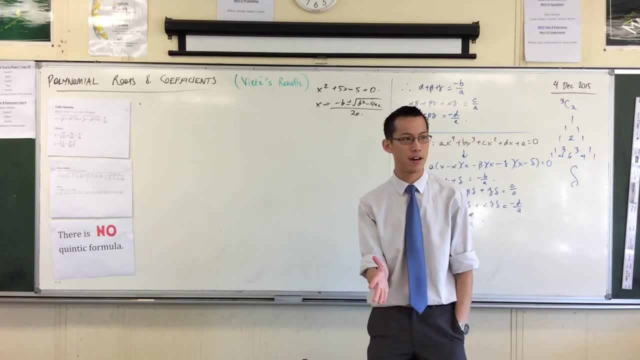 Five and above, a formula can't be found, It doesn't exist. Now, this is um. you're probably guessing. you know we're going outside the syllabus, but I do want to say to you, right, Um, these methods here- one, two, three, um they're what we call um algebraic computation, right? 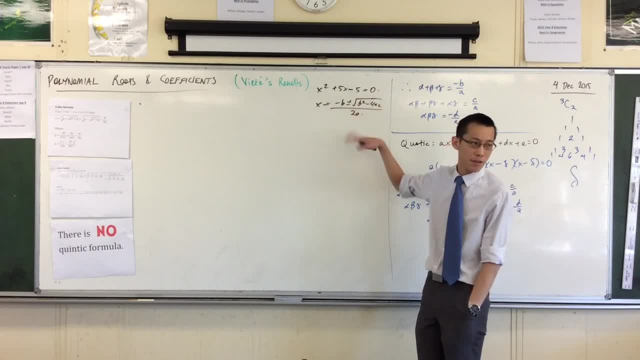 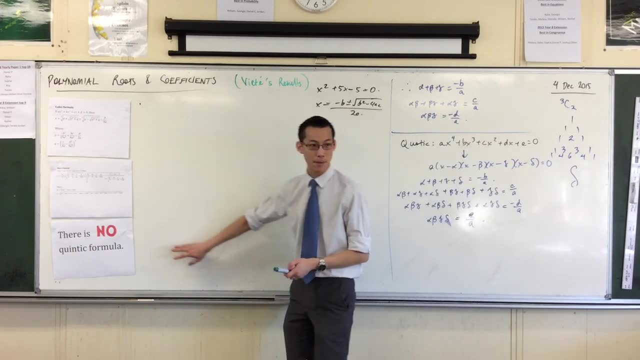 Like what is algebraic computation? We're using tools of algebra Like these are all algebraic: Plus minus square root, squaring. that's all algebraic operations. right, If you want to find the roots of anything above this, or even practically speaking, 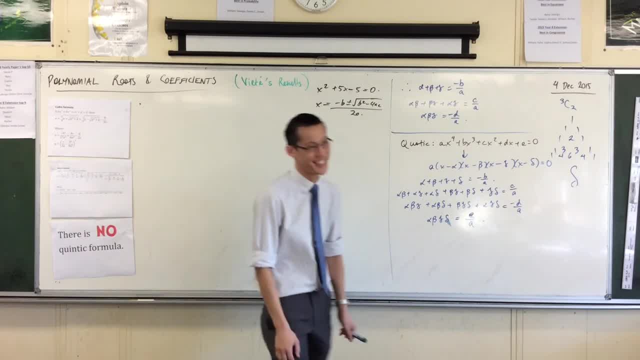 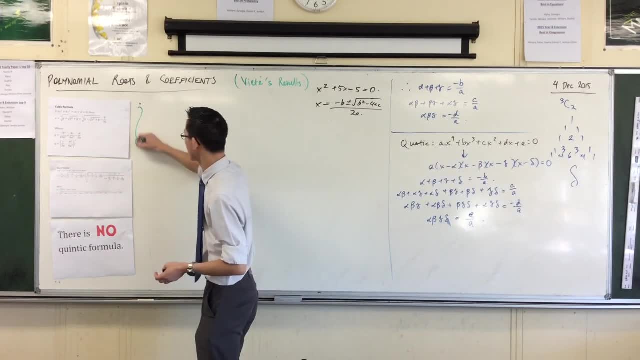 if you want to find these roots, like these formulas exist, but no one uses them, right, Because look at them like you can't even read that thing. okay, Instead of doing that for anything kind of like this, we use methods called numerical approximation. 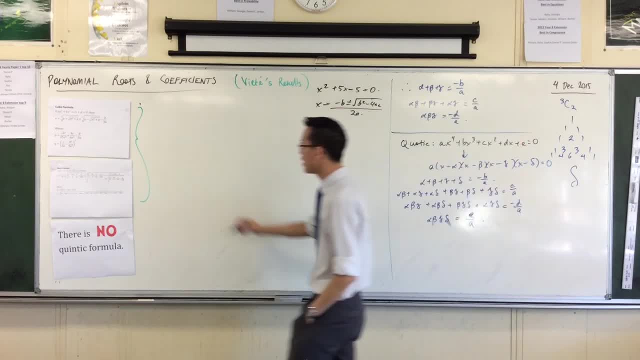 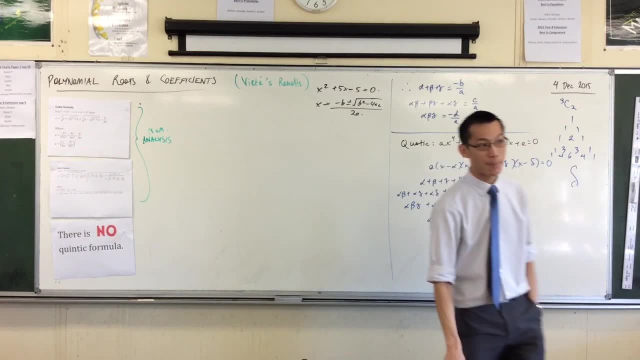 Uh, it's in a field of mathematics called analysis. okay, So analysis, And we're actually going to next year, numerical analysis- We're going to learn um a couple of methods for approximately finding what the solutions to these equations are. 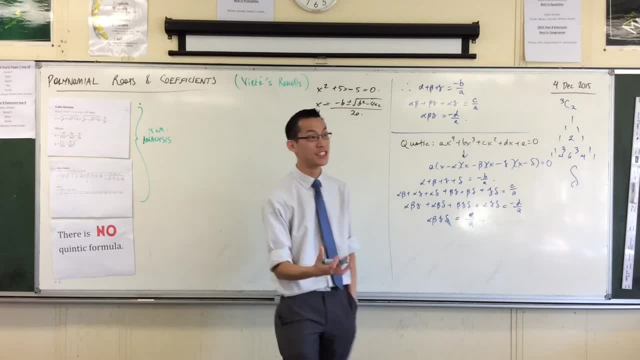 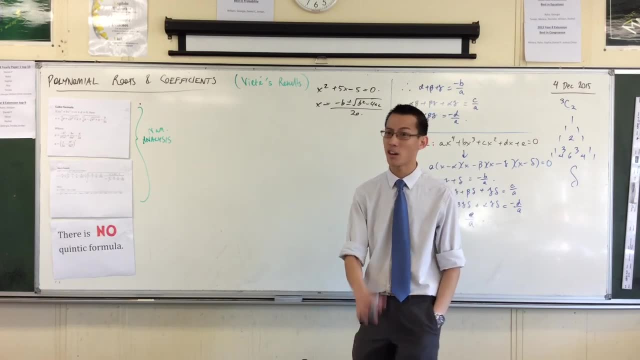 Because finding them exactly is ridiculous, Like it's legitimately ridiculous, right And um, if you want to find an answer for these things, you just need to get close enough, Like get me five decimal places and that'll be accurate for any building or any like architectural or any physical application you want. okay. 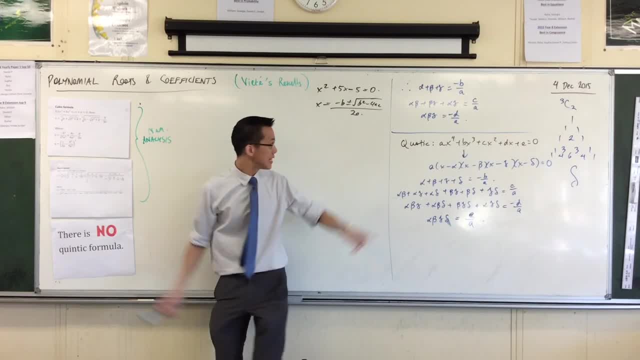 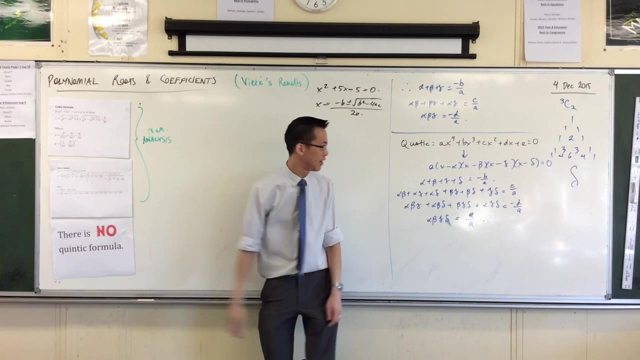 Um, but this is just astonishing that we can work with Like these things. see these simple, simple numbers that you get out of here, The numbers you're adding up and multiplying. are these numbers right? And we reduce something that's insane and so so difficult that we invent a new field of maths to work with them. 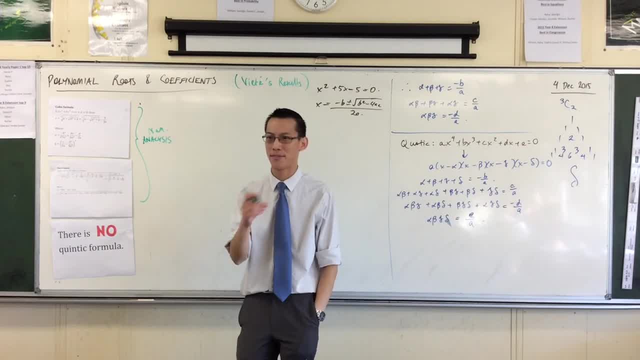 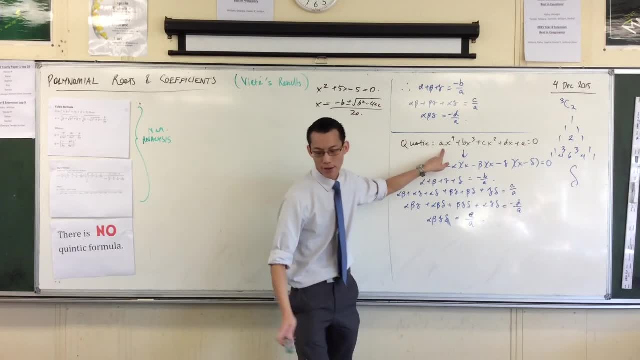 You just have to like divide some numbers. That's all you have to do. Does that work for? um, like paintings, This, these results. they just keep going right. Oh right, I could. I could vary. 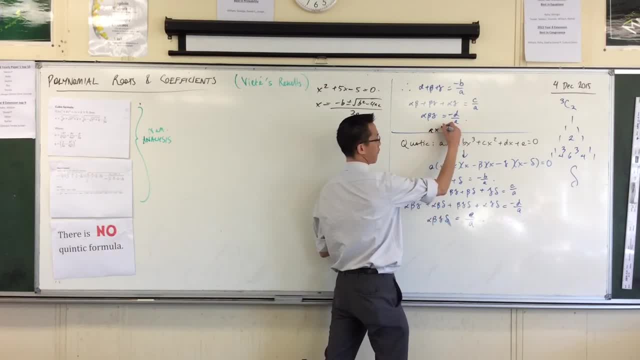 You won't. But I could very easily write, you know, ax to the 5 plus bx to the 4, da-da-da-da-da, right. And then over here you'd have x minus alpha, x minus beta, x minus gamma, x minus delta, x minus epsilon would be the next one.